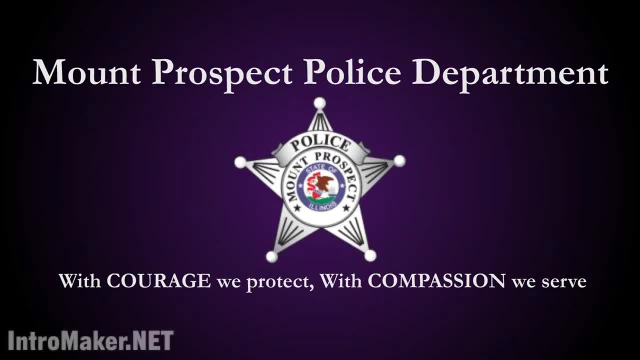 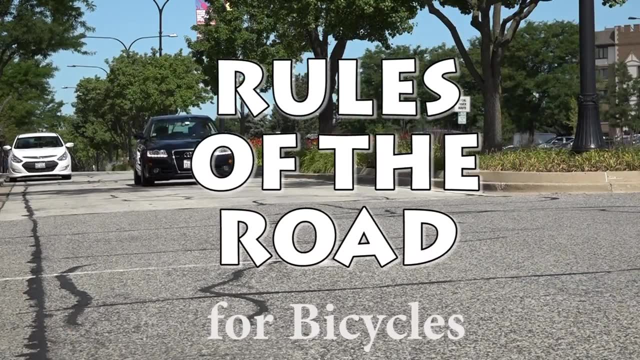 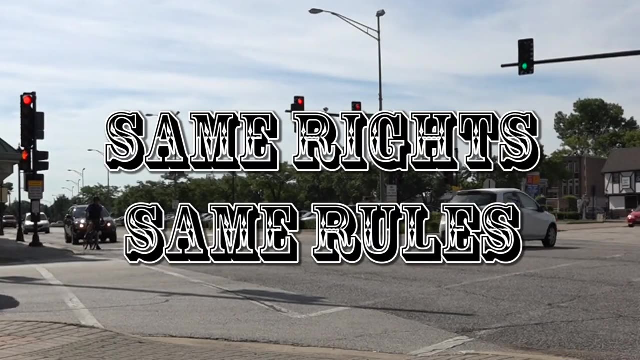 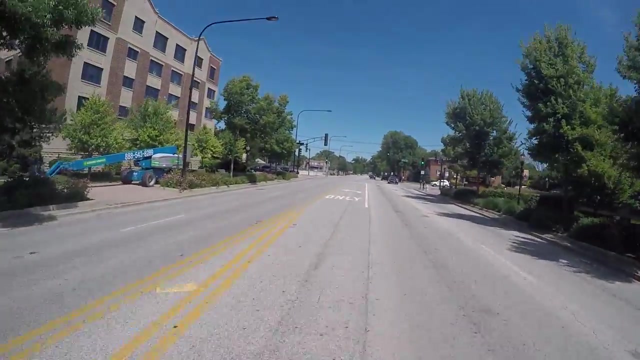 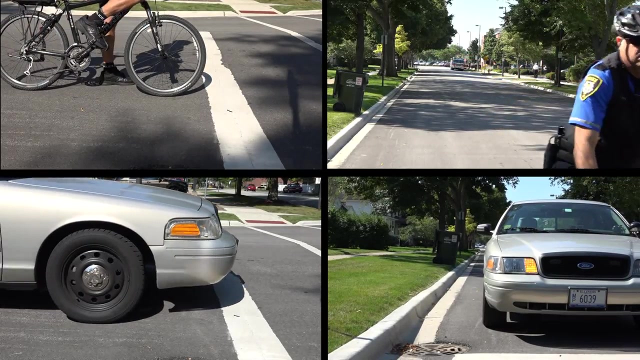 To get around town in Mount Prospect. here's what you need to know about the rules of the road while on a bicycle. Did you know that people biking have the same rights and the same rules as people in cars and trucks? A bicycle riding on the road is considered a vehicle in Illinois and riders must obey the same traffic laws, signs and signals that apply to motorists. 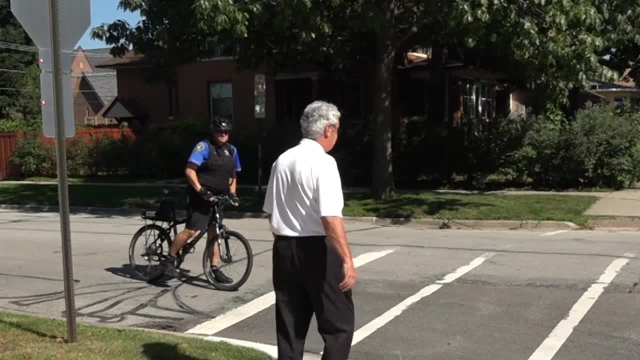 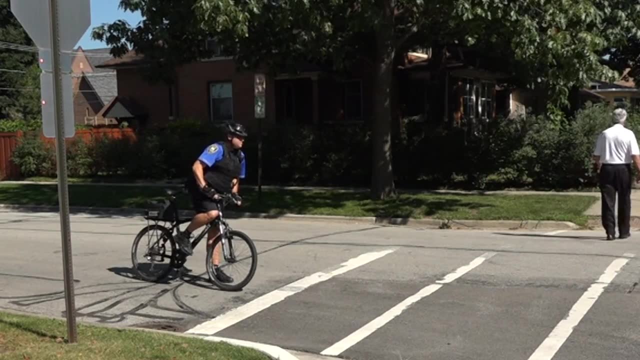 People walking have the right of way, so please watch out for them when you are biking. Right of way laws apply to bicycle riders, motorists and pedestrians. If others do not follow the rules, let them have the right of way to avoid the risk of a collision. 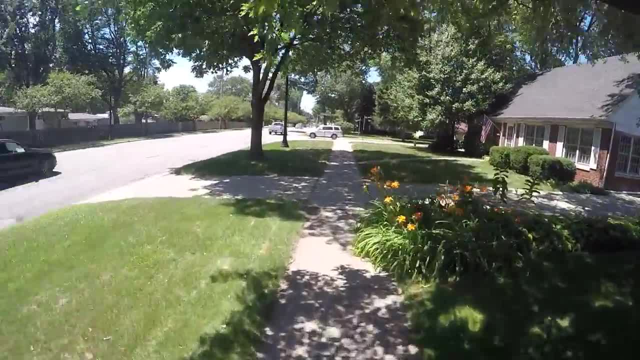 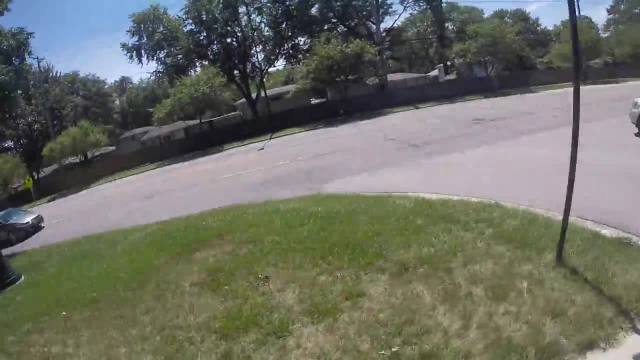 The National Highway Traffic Safety Association recommends children less than 10 years old ride on the sidewalk. While it is legal to ride on the sidewalk in Mount Prospect, it is safest to ride on the street. Bicyclists must yield the right of way to pedestrians and give an audible signal when approaching 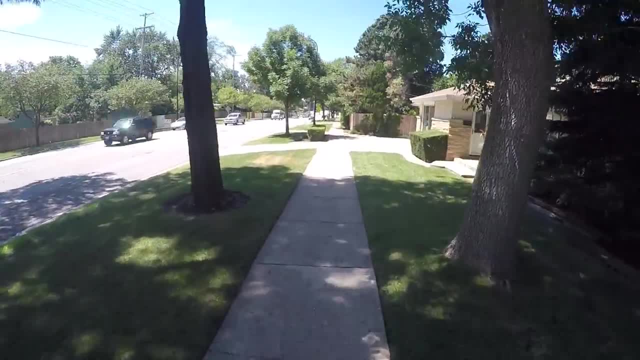 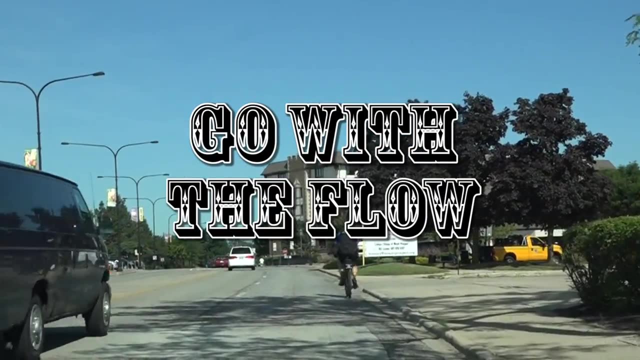 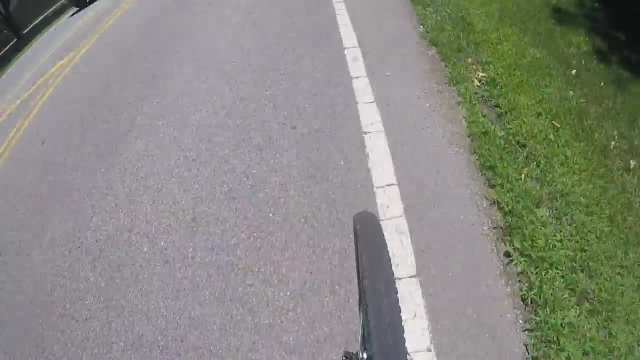 You can also see pedestrians approaching a pedestrian from behind to alert them of your approach. Ride on the right side of the road in the same direction as other vehicles. Riding in the opposite direction of traffic is not only dangerous, but it is against state law. 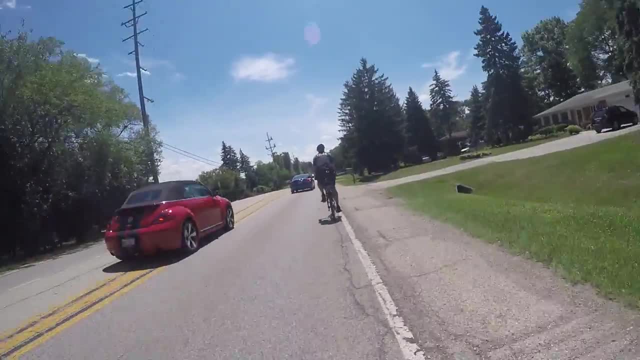 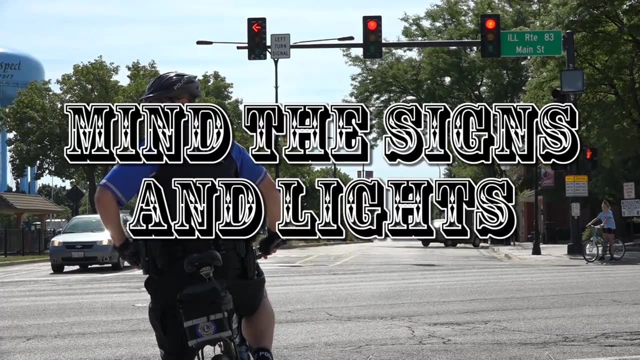 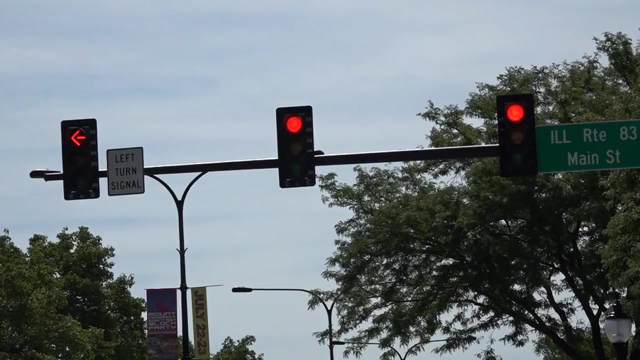 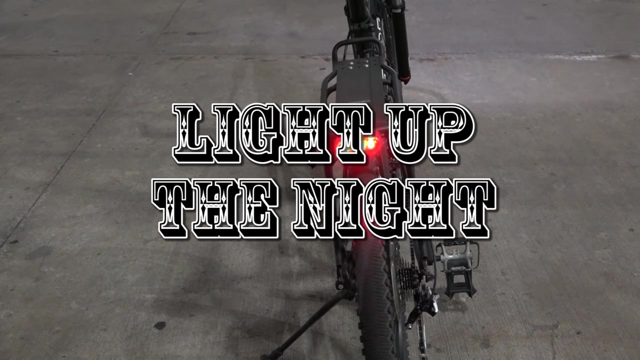 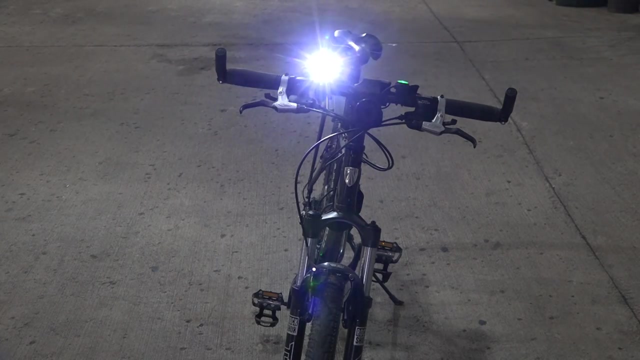 Motorists are required by law to allow at least 3 feet of space between them and a bicyclist while passing. Just like all other vehicles, you must stop at stop signs and obey traffic lights. If you are riding at night, state law requires your bike have a front light visible from a distance of at least 500 feet and a rear red reflector visible for up to 600 feet. 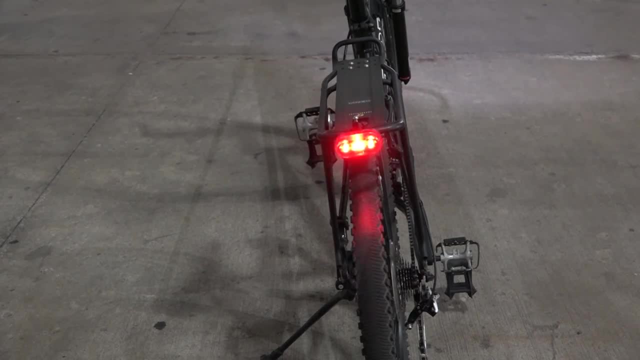 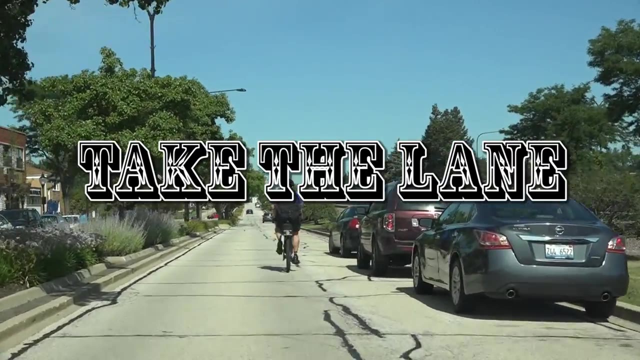 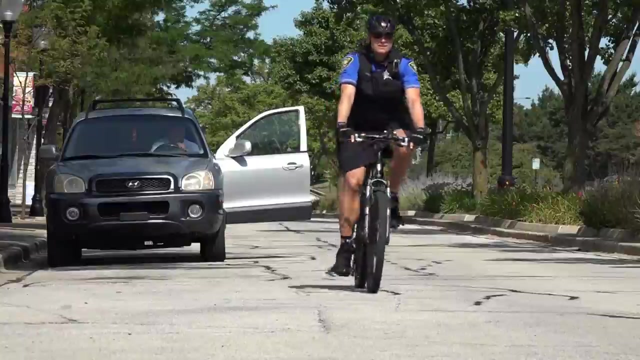 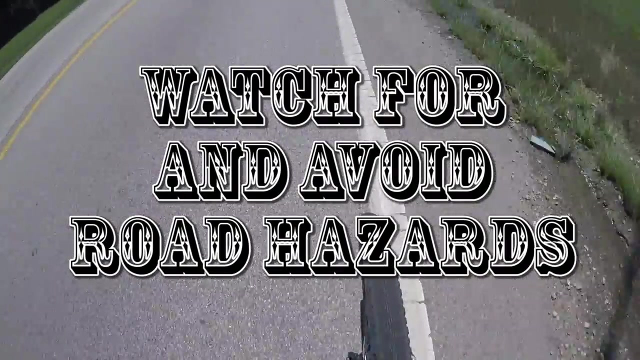 Always wear white and or reflective clothing when riding at night. Also, make sure to wear a mask while you are on the road. On narrow streets, take the lane to avoid riding in the door zone. Listening to music while riding might be fun, but be sure to be able to hear oncoming traffic by having an ear clear.